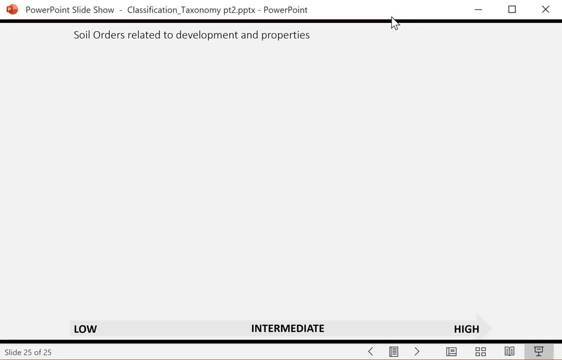 you notice across the bottom, we've got some ideas that soils have different degrees of development. They also have different properties, and so this one looks at the amount of development and those properties, And in thinking of development, we're thinking about what factors actually limit the development of a soil profile. So with an entosol, that's material, that's. basically recently been deposited or recently been weathered. from the bedrock that's in place, There's been very little time for development to occur or the weather conditions that have been in place inadequate for development to occur. So these are new soils. 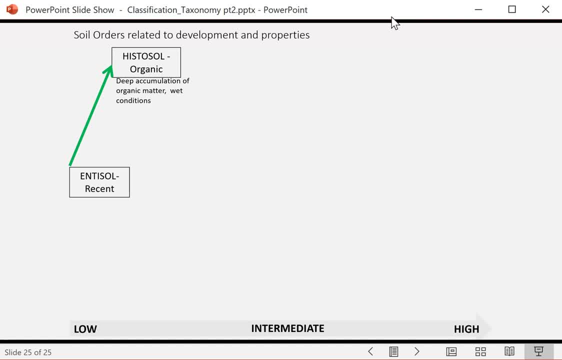 Now, when you get to a histosol, the amount of profile development is limited, primarily because of the conditions under which that histosol develops, which are: there's a lot of organic matter, but the wet conditions limit the decomposition of the organic materials, the plant residues. 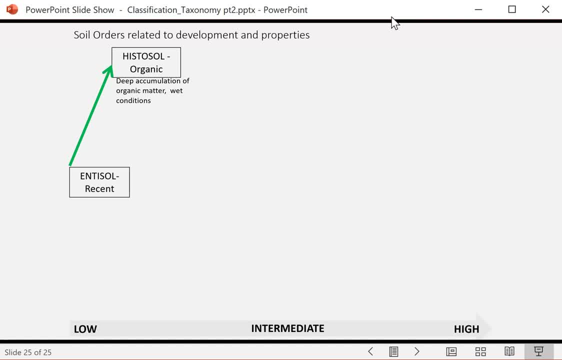 and things that are deposited in the water. The decomposition is slow, but that also means that there's not a lot of development in the profile below that. once you get into the mineral portion, Gelisols, it's too cold for much soil formation to occur. 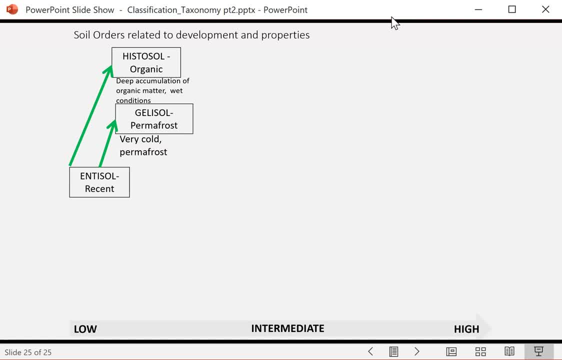 because there's permafrost at some depth in the soil. Now, this: typically you'll find these in extreme latitudes- north and south Canada, Alaska, or northern Canada, Alaska, and then the other thing is parts of. 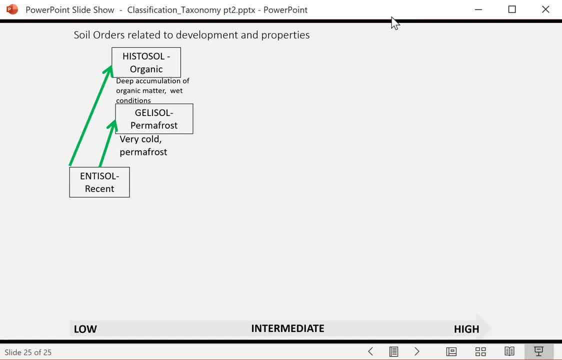 Russia, Siberia, but the other issue there is- you can also find those in. there are montane or mountainous regions that have the gelisols when you get your elevation high enough and the soil never thaws below some depth, and that's also why trees don't grow above certain levels. 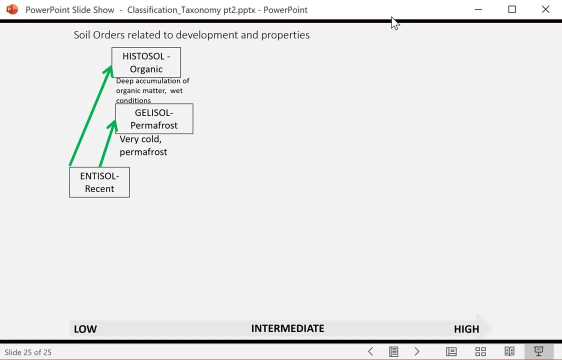 in the mountains because you get to a point where the soil is frozen and the tree roots can't grow through them. Enceptosols: these are just a little bit of a difference. They're a little bit older than the entosols. 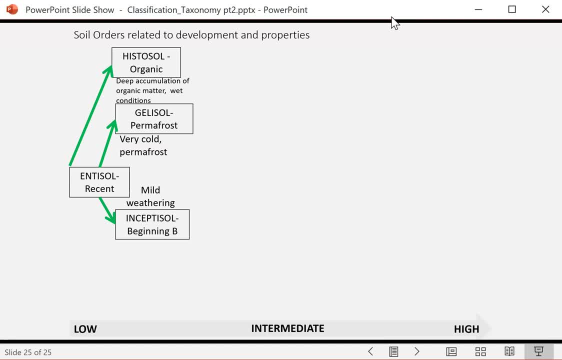 Soil formation has started, but they haven't been on a stable landscape for a long time. They haven't been there a long time. The conditions in the weather- weathering and soil development conditions- have not been sufficient for much development to occur. Entosols- materials that are deposited. 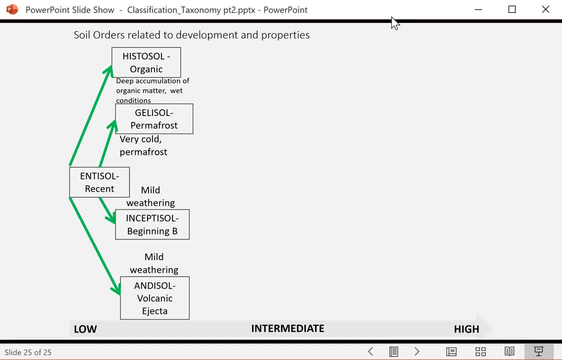 through volcanic ejecta if there's not been a lot of weathering occurring in those, and those have some really unique weather minerals in them that tend to limit a lot of development. Once you get into more development, you move into other soil orders. 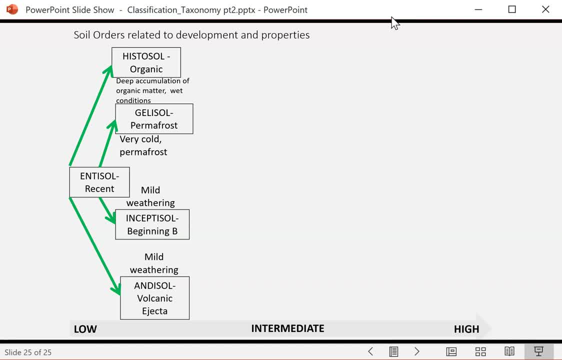 and so these entosols are kind of on the young order of materials that were deposited by volcanoes. So then we go to our next level of things that have some degree of intermediate development. I mentioned earlier that erytosols may have developed in conditions other than the current climate. 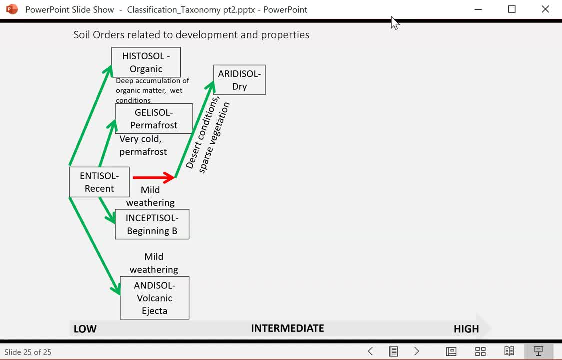 but they're classified based on the climate that they are in now, And so the profiles that you see are kind of very widely, and probably many of these have no current soil development occurring. You've got desert conditions, you've got sparse vegetation. 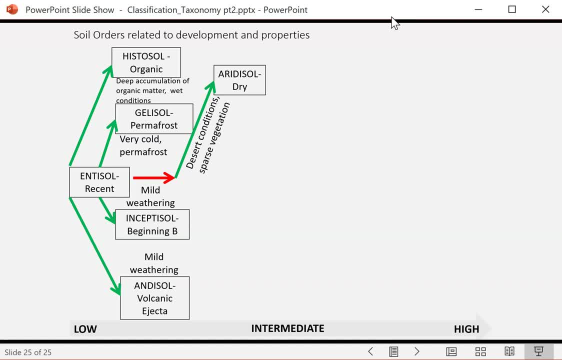 and in those cases the dry is the thing that's the chief characteristic for diagnosing or classifying an erytosol. Then in the desert you've got desert conditions and if you have, soils with a great degree of shrink-swell, 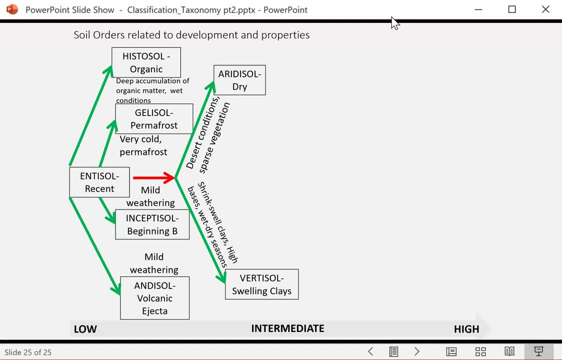 the high base is that base saturation. So they're alkaline, or at least neutral to alkaline soils. They're not acidic and they have distinct wet and dry seasons, which is what allows those soils to shrink during the dry season and swell during the wet season. 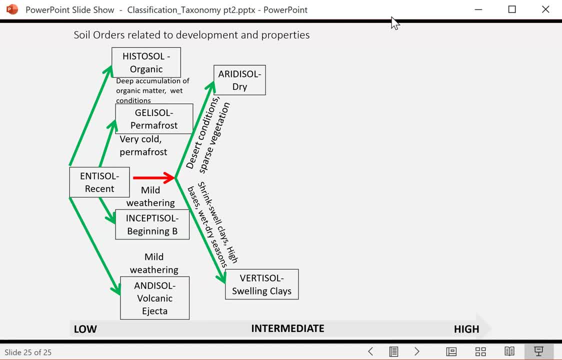 and they develop some interesting and unique characteristics, like the slickensides we've mentioned in the other, which is the version of the key that help us recognize those, And the churning in that soil associated with those shrink-and-swell cycles limits the amount of soil development. 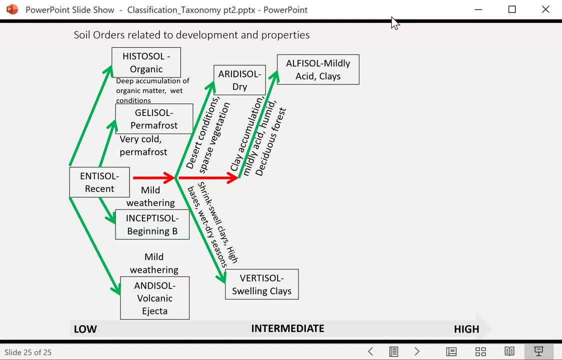 Now you increase, go up another degree on the amount of soil development. You get these alphasols. Those are associated with deciduous forest primarily, although you can find them in other places. They've got some clay accumulation and the B horizon. they're generally slightly acidic. 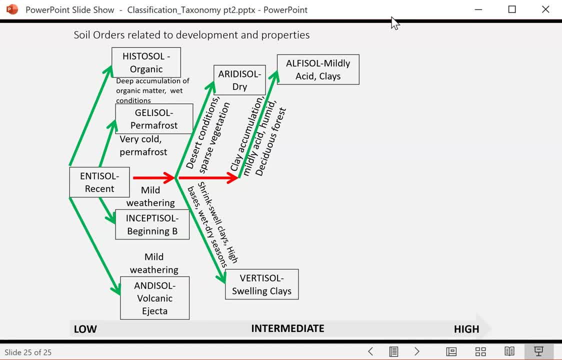 in those deciduous forests in that region. In other places they might not be, because the formation conditions are different, such as the sandy loam surface alphasols that exist in the southwestern Great Plains. The conditions: sand doesn't allow it to accumulate the organic matter.